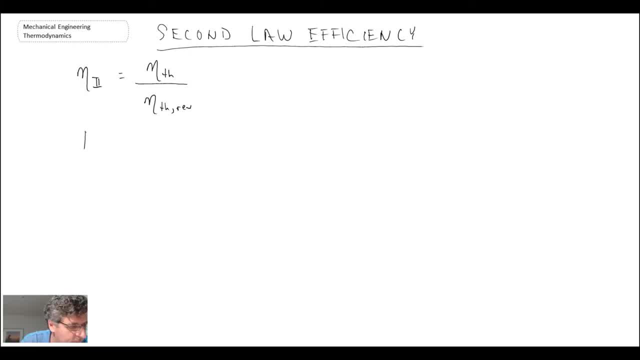 So the second law efficiency can be defined as: So the second law efficiency can be defined as being the thermal efficiency of the cycle that we're looking at. So what we can say is that the second law efficiency is a ratio of the thermal efficiency of an actual heat engine to that of a reversible heat engine. 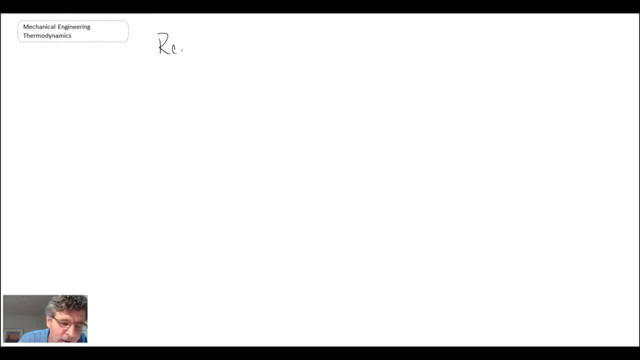 Another way that we can write the second law, efficiency is if we look at what exergy itself is. Let's compare the thermal efficiency to the total heat efficiency of a basil Ericksonian aquelesquare circles versus a steel, that which is equal to the thermal efficiency of a heat Под 1500. 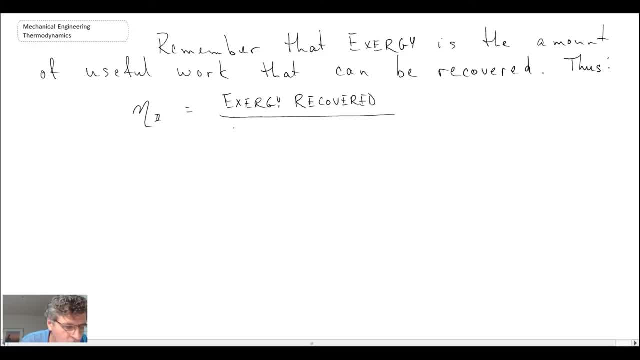 So in that case for an exergy analysis, exergy evaluations are: guerrillas have built itself from coolant with a heat chance of mojequpetite feet are mini ball. So under this, assume that exergy analysis is not complete enough to evaluate the total heat efficiency of a basil ericksonian. 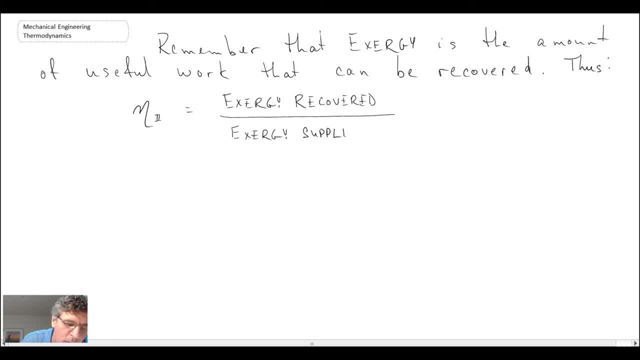 So another way to think about this in terms of exergy itself is the second law: efficiency is the amount of exergy that we are able to recover divided by the amount of exergy that is supplied at a given state. So if we're going to 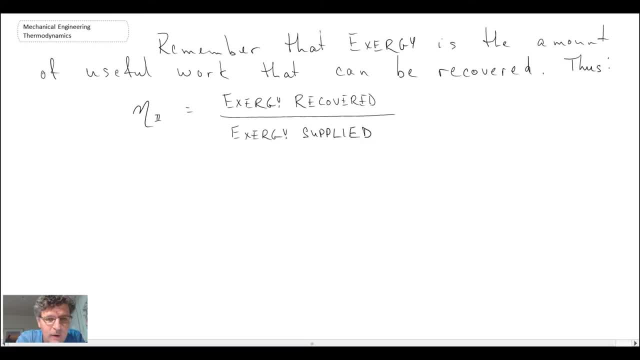 examine exergy and we want to be able to determine the amount of exergy, like we looked at when we looked at the temperature supply or the source of 1500 Kelvin. what we need to do is come up with a useful method of being able to